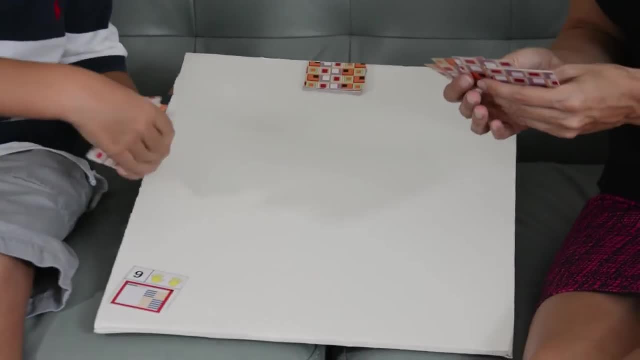 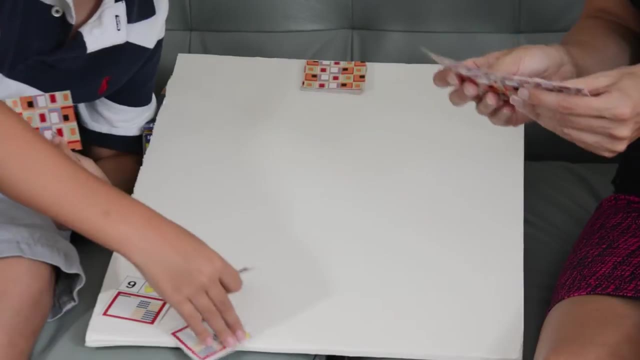 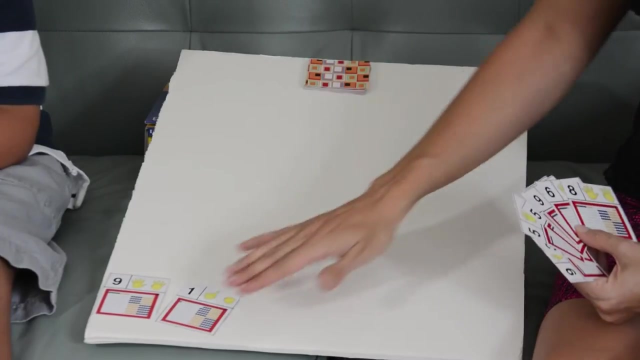 It can be either two cards that add to ten or three, Or you can make subtractions Or a mixture of subtractions and additions. So the object of the game is to collect the most cards by doing equations. So superhero here, put a nine and a one. 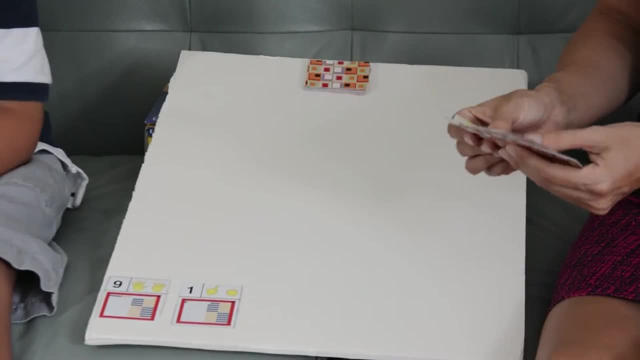 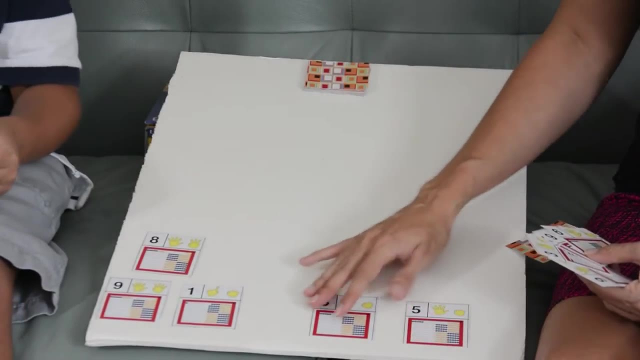 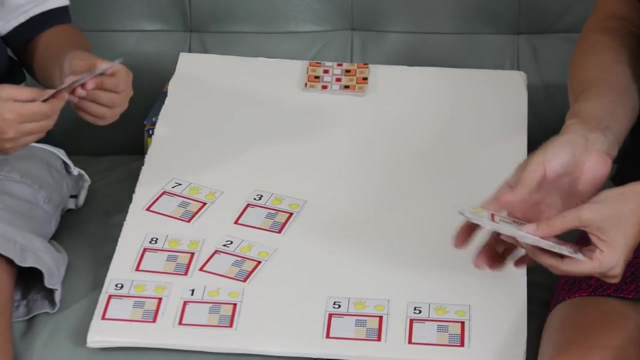 What is the equation? Nine plus one makes ten, Perfect, so I'm going to do one, two And we need to do the one that does the most cards wins, And you just need to continue to replenish your hand by drawing from the deck. 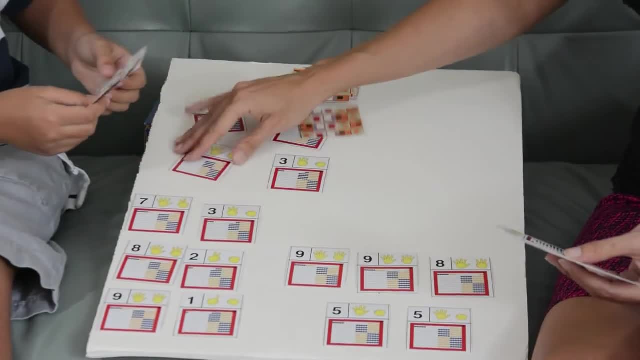 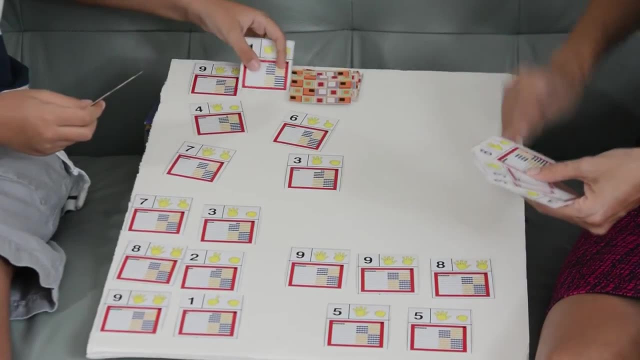 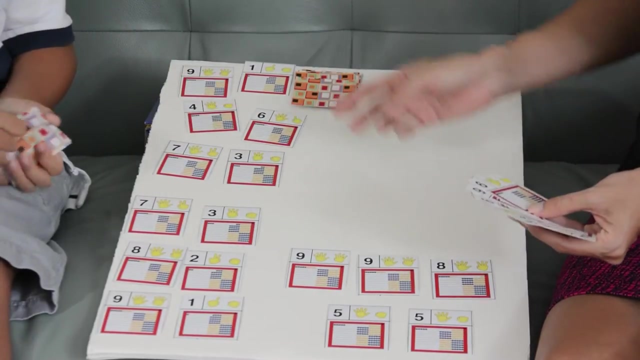 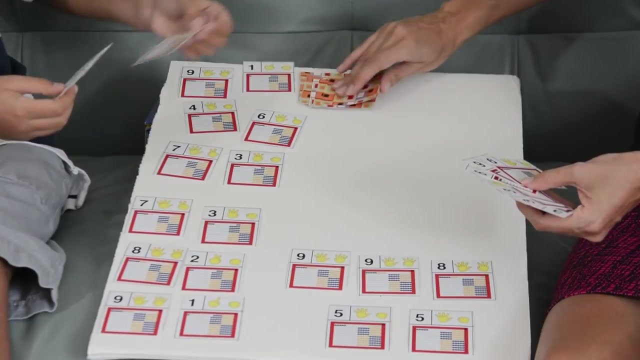 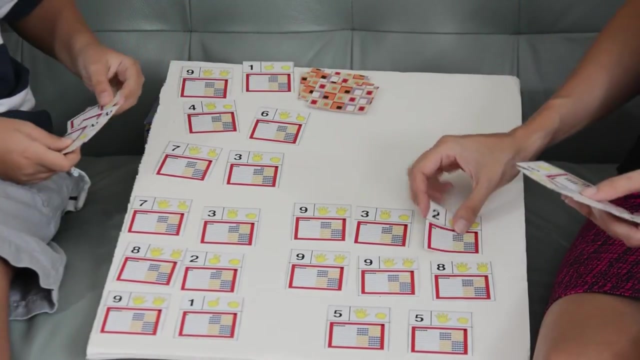 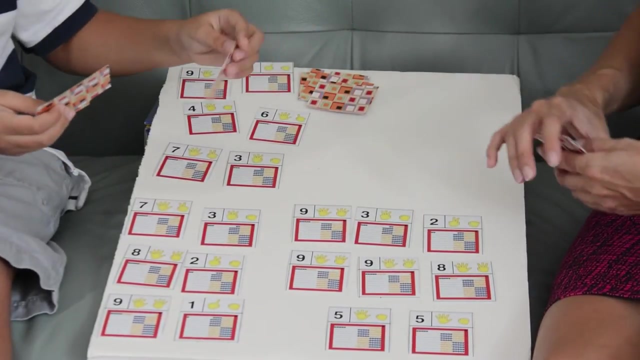 So each line here represents an equation, But you can continue. I don't have anything here. You have to get something, Ok. so there I have one more. Nine plus three equals two equals 12. minus 2 equals 10. and we will continue to do that and fill up our 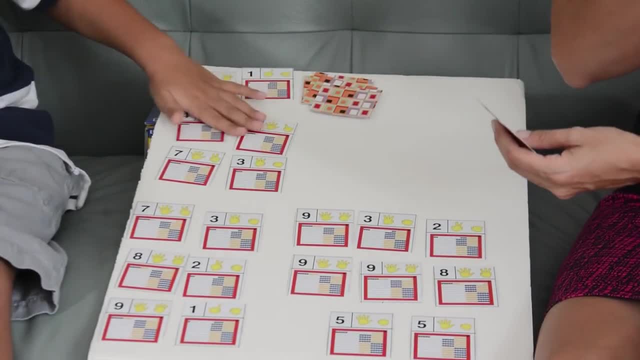 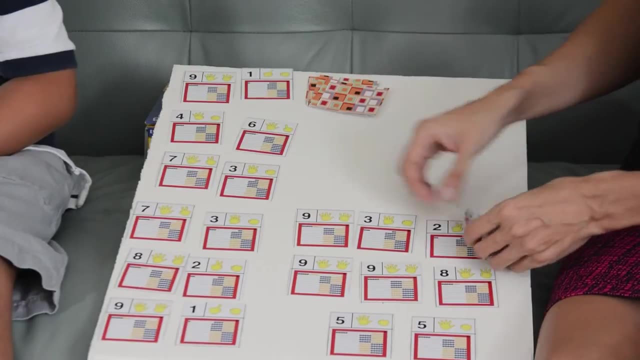 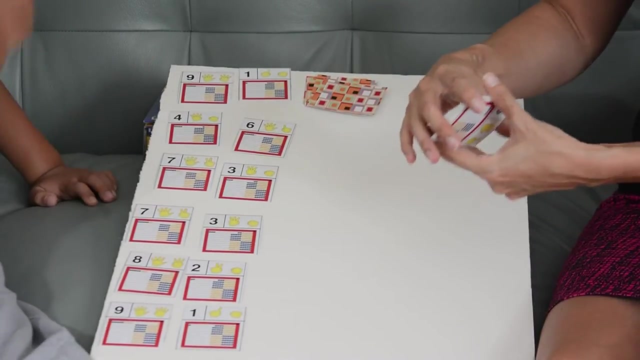 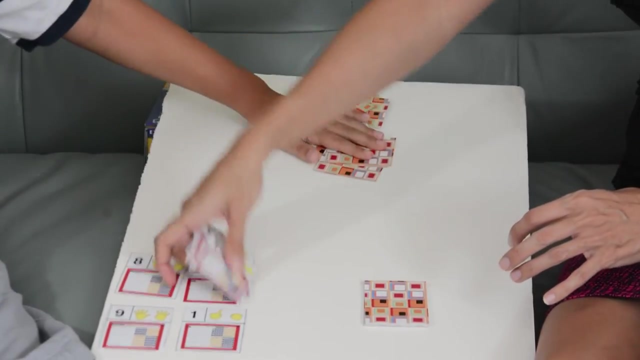 table with equations, and then the person who collects the most cards at the end of the, once the deck has been exhausted, is the one who wins. and, as usual, we just make sure first that all the equations are correct, and then we know who's who's the winner. we're just stacking the each of one, each of our decks, next to each. 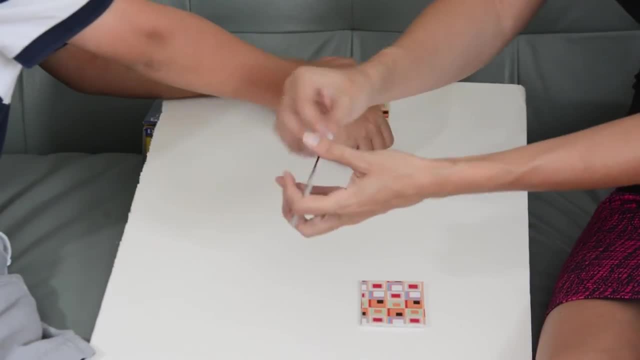 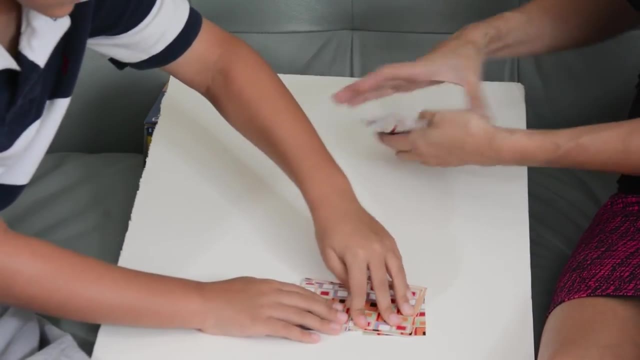 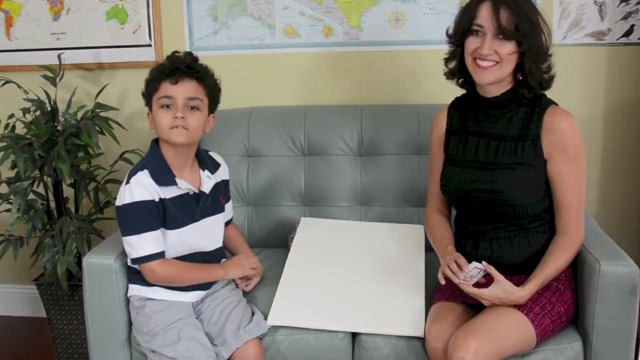 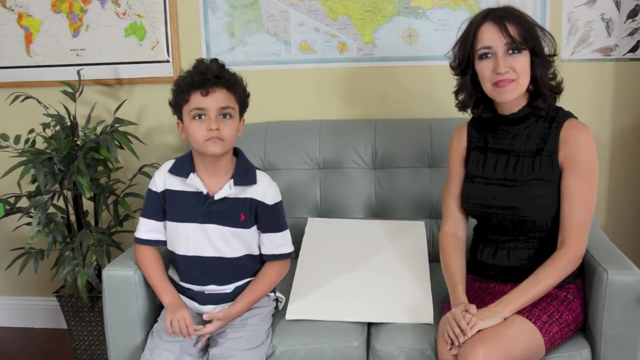 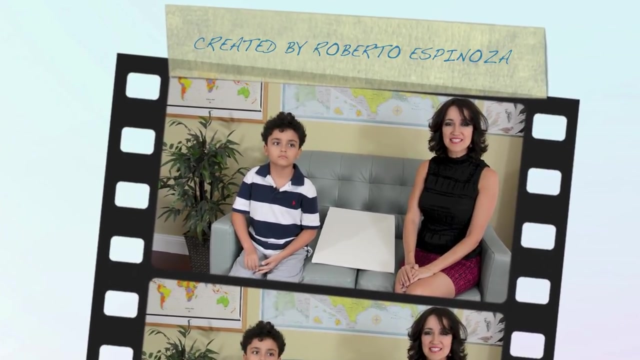 other. that way we don't have to count. so that's it, that's today. I hope you had a good, a good time playing. go for ten, bye, bye. to learn more about math games, please visit our website at raisingaselfreliantchildcom and also please remember to rate and subscribe. thank you.